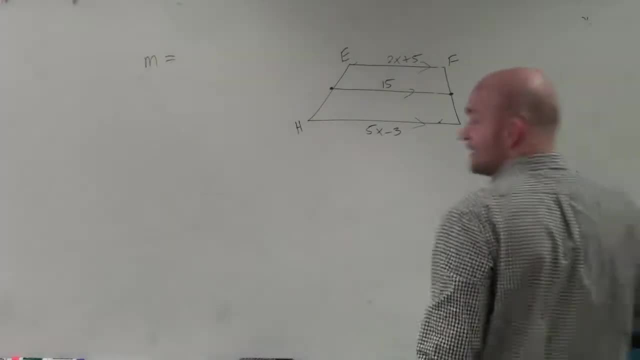 OK, So let's try that again. So in this case, what they're trying to ask you to do is to find x. Now, remember, this is a trapezoid, they tell us, And they also say: we have a mid-segment which. 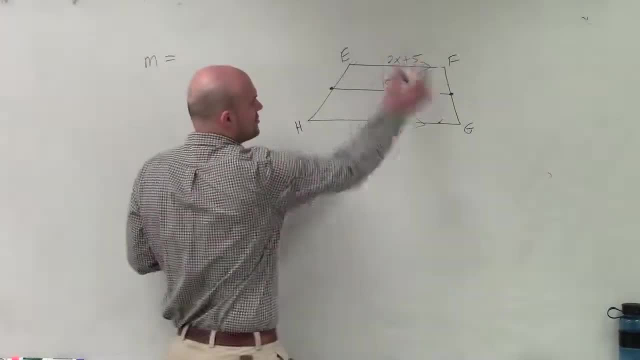 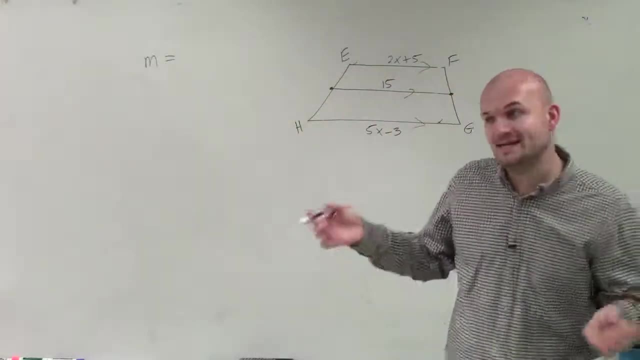 is the length of 15.. Now, in this case, we know that these two are parallel, as well as our mid-segments, But we need to go. what is our mid-segment formula? How do the bases and the mid-segment relate to each other when it's a trapezoid? 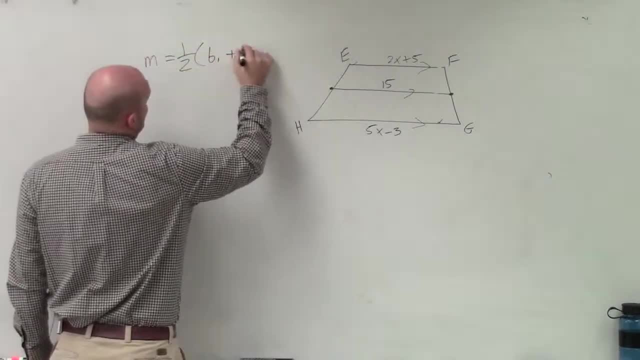 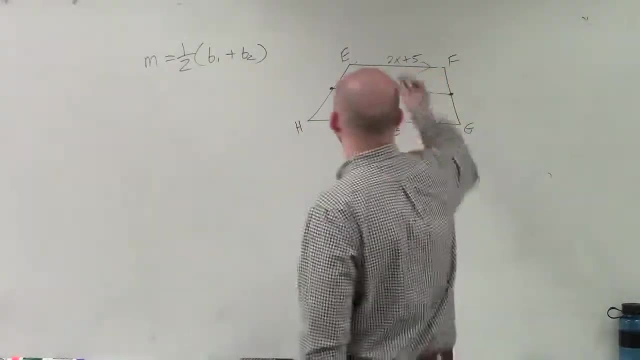 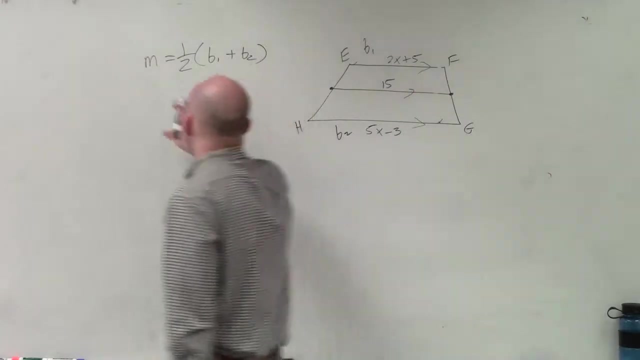 So that formula is the sum of your bases times 1. half is equal to the length of your mid-segment. So it doesn't really matter what your bases are, but I'll call that base 1 and that base 2.. So if we look, do we know the length of our mid-segment? 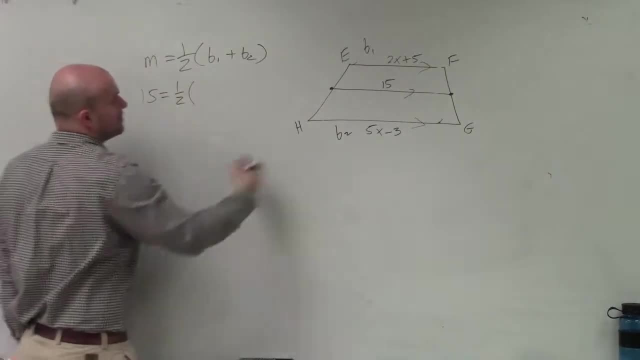 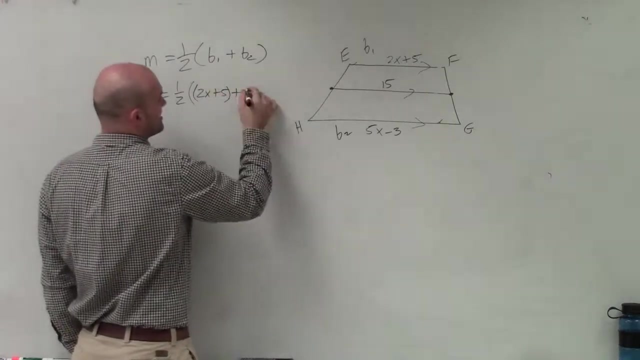 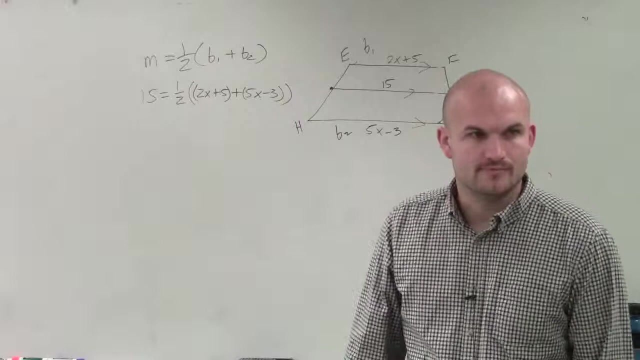 15 equals 1 half base 1, I'll call 2x plus 5, plus 5x minus 3.. Yes, Does that make sense? You're adding your bases. We don't have numbers for the bases, we have expressions. 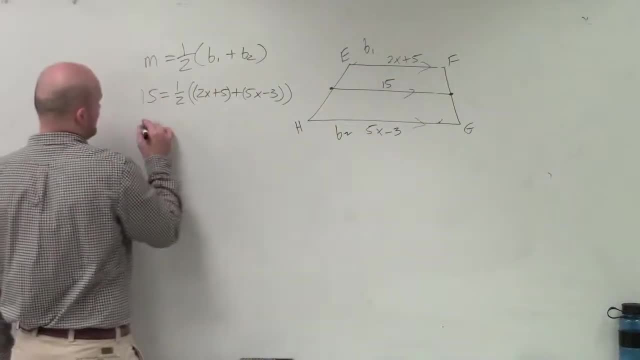 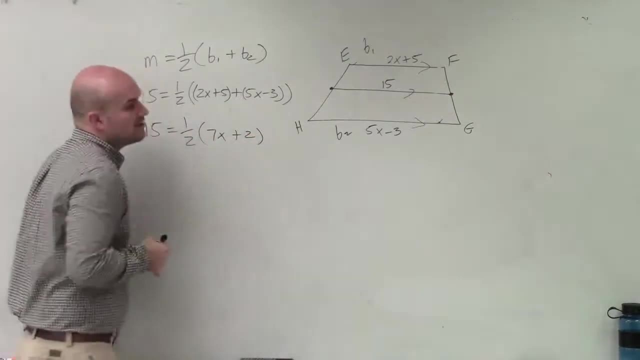 But that's OK. So now I can combine like terms. So I say: 15 equals 1 half, 2x plus 5x is 7x plus 2.. Now to solve for this, you could distribute the 1 half. 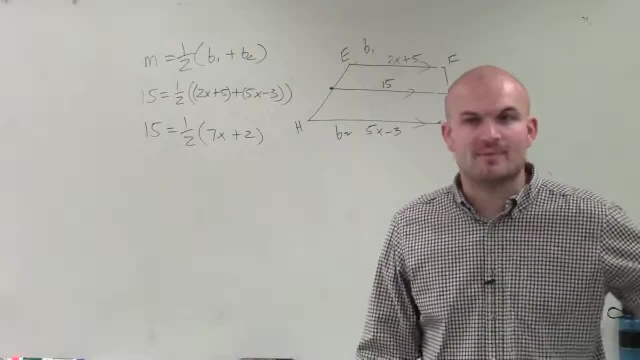 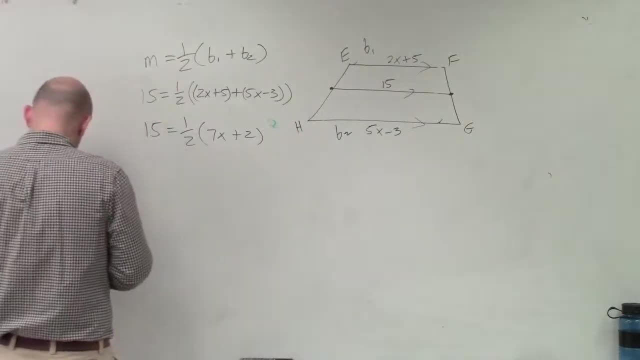 if you'd like to. I don't like distributing the 1 half. I like to multiply by the reciprocal on both sides, So I'll multiply by 2 over 1.. Oh, I'm awesome. So I'll multiply by 2 over 1.. 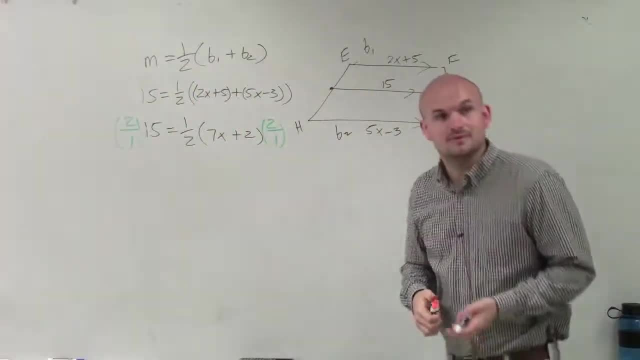 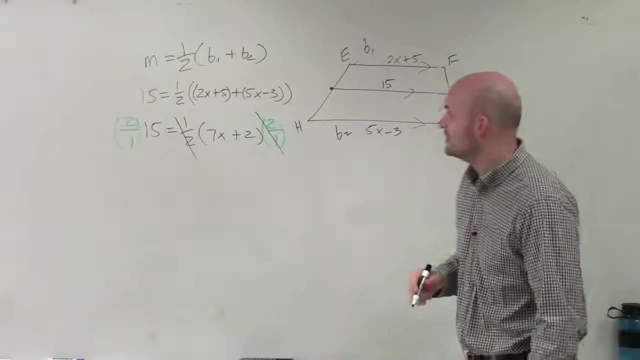 It's called the no-look pass Devin. Huh Yeah. So thank you, Jake, for your comment, but I don't think it's needed. But I appreciate it. So we can multiply by our reciprocal Obviously any number multiplied by its. 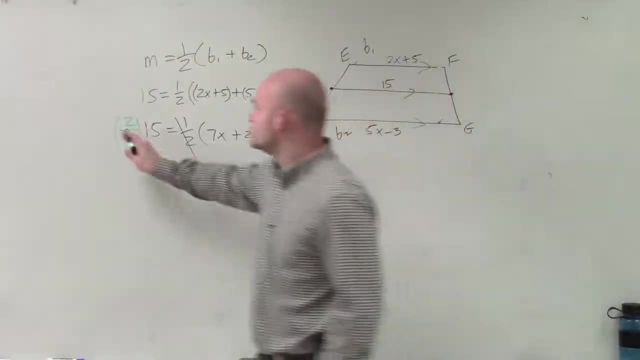 is going to be a 1.. So that's just going to leave us with 7x plus 2.. 2 over 1 times 15 is going to be 30. Or 30. Or 30. Or 30.. 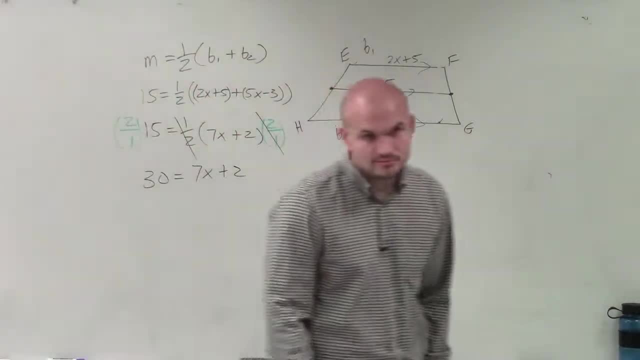 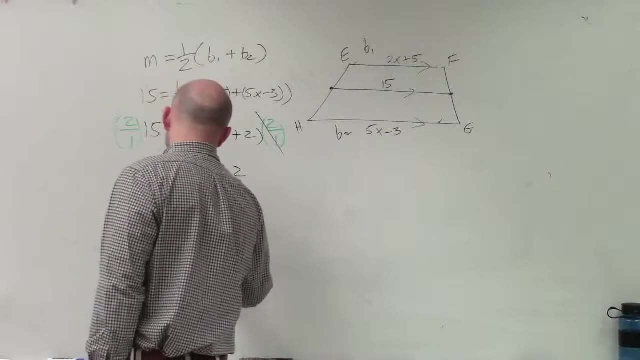